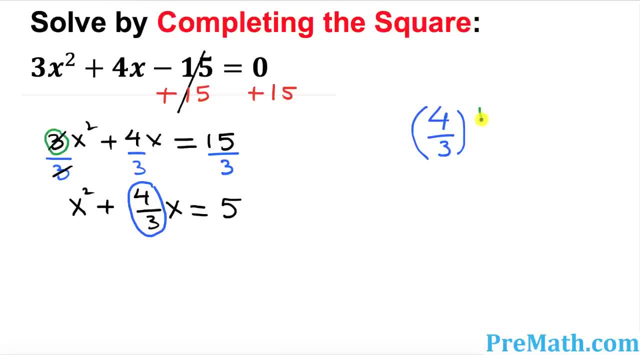 the half of this number is simply by multiplying by 1x over 2. so once you do that one, that's gonna give you what 4 times 1 is 4, and on the bottom, 3 times 2 is 6. I want you to reduce this fraction that turns out. 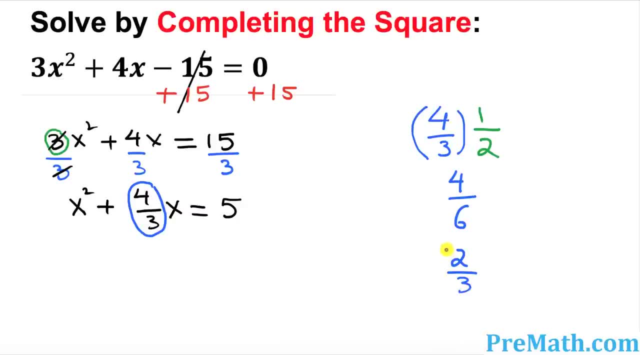 to be what? 2 over 3. and now, whatever you got, you must take the square of this one. once again, what we did, we took the coefficient of this X, which is 4 over 3. we want to take the half of this one. it's the same as multiplying by 1 over 2. 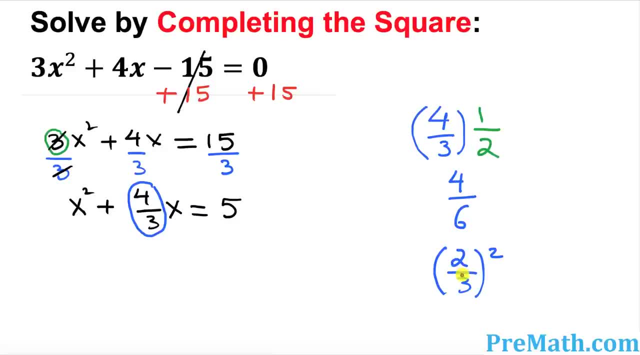 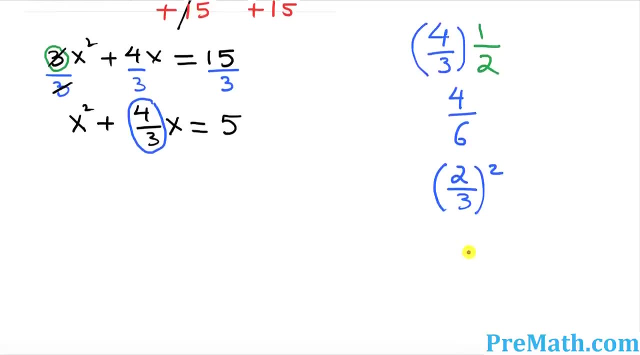 we got 4, 6 and it reduced to what? two-thirds and 10. then take the square of that one, so we're gonna add this quantity on both sides of this equation. so let's go ahead and do the next step: x squared plus 4 over 3x plus, and I'm gonna 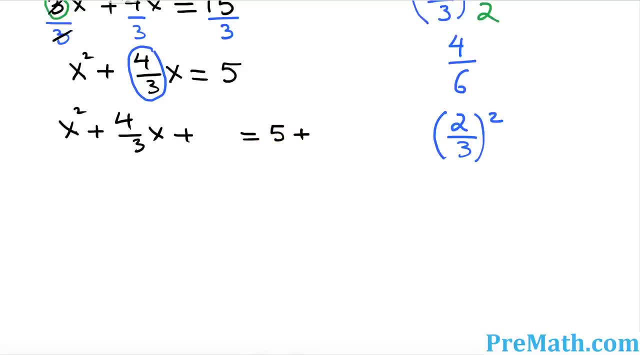 put down 5 plus. now I am going to write down this: 2 over 3 squared on this side, and 2 over 3 on this side as well. now you can see this left hand side is a complete square of what? X and then the plus sign in between this one and this 2. 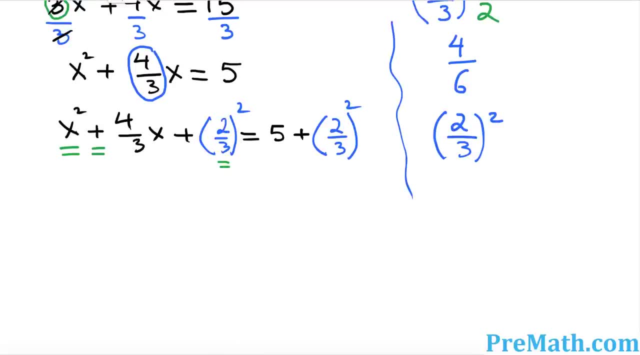 over 3 inside this parentheses. so let's go ahead and write it in this parentheses X, and then this plus sign, and then this 2, third only, and then complete square power. 2 equals to 5 plus 3 over 2. square is simply 4 over what, 9. 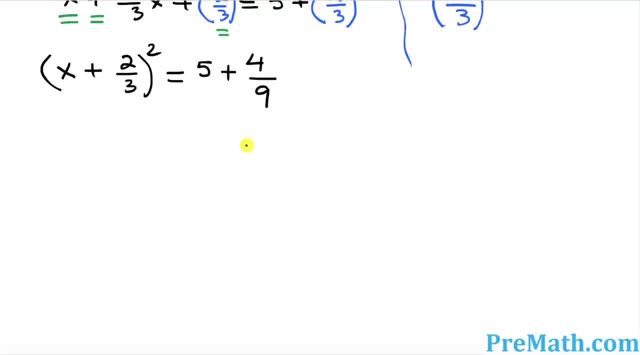 so the next thing we, what we want to do is: I want you to add these, I want you to add these. I want you to add these two quantities: 5 plus 4 over 9. I'm going to write down over here: 5 could be. 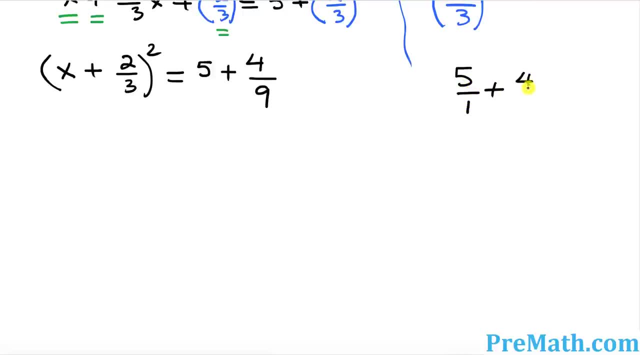 written as 5 over 1 plus 4 over 9. so we're going to add these two fractions. so the simplest way is just simply: cross multiply 4 times 9 is 45. then whatever this sign, you just put it there and then cross multiply this one again. that's. 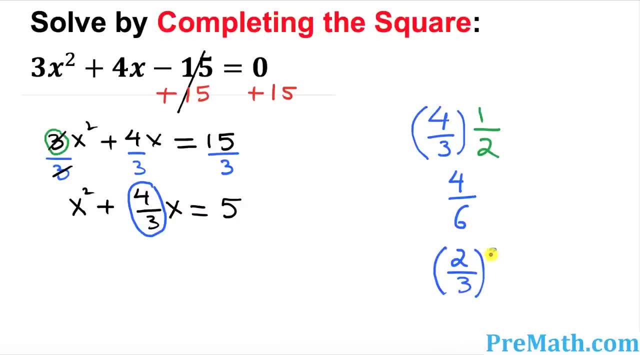 whatever you got, you must take the square of this one. Once again, what we did: we took the coefficient of this x, which is 4 over 3.. We want to take the half of this one. It's the same as. 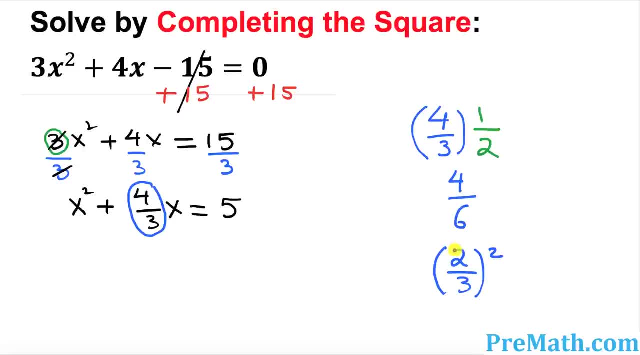 multiplying by 1 over 2.. We got 4, 6 and it reduced to what? 2, third and 10.. Then take the square of that one. So we're going to add this quantity on both sides of this equation. So let's go ahead. 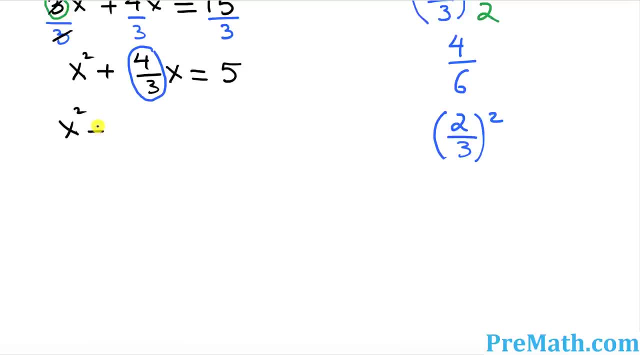 and do the next step: x squared plus 4 over 3x, x plus, and I'm going to put down 5 plus. Now I am going to write down this: 2 over 3 squared on this side, and 2 over 3 on this side as well. Now you can see this left hand side is a complete square of what x and then the plus sign in between. 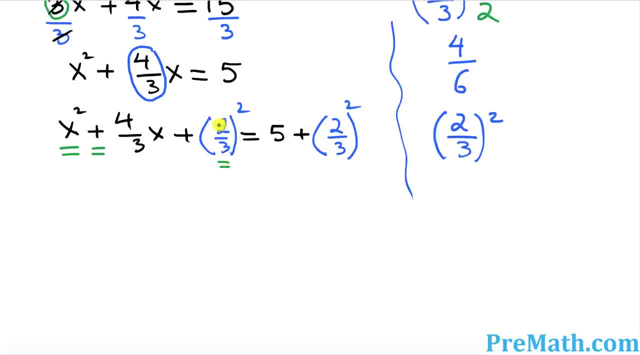 this one and this 2 over 3 inside this parenthesis. So let's go ahead and write it in this parenthesis x, and then this plus sign and then this 2, third only, And then complete square power. 2 equals 2 times 3 over 2. squared is: 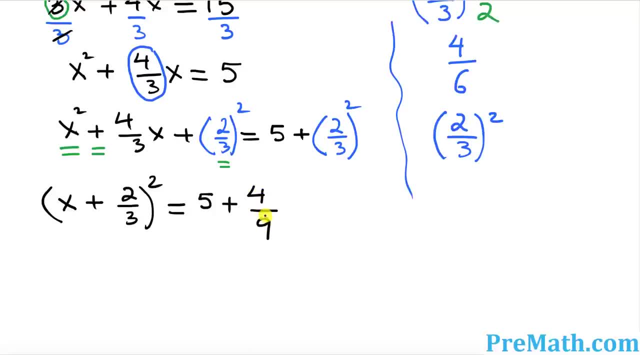 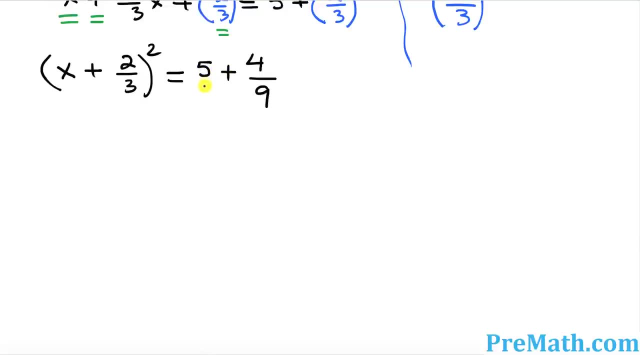 simply 4 over 9.. So the next thing we do, what we want to do, is: I want poka, poka, poka, poka, poka. who-jo want you to add these two quantities: 5 plus 4 over 9. I'm gonna write down over. 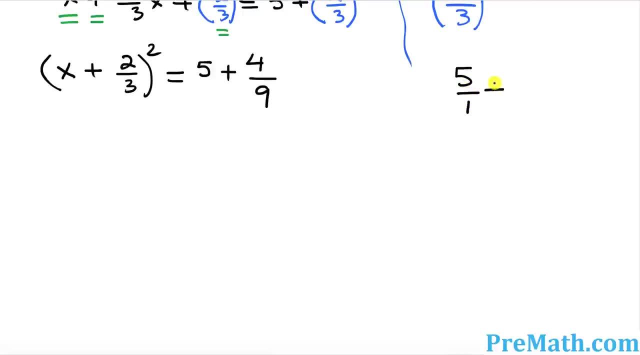 here, 5 could be written as 5 over 1, plus 4 over 9, so we're gonna add these two fractions. so the simplest way is just simply cross multiply 4 times 9 is 45. then whatever this sign, you just put it there and then cross multiply this one. 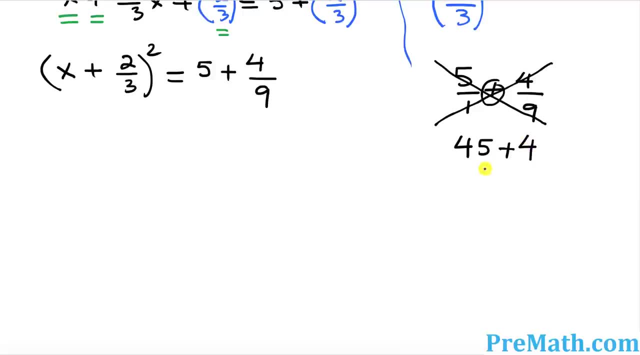 again. that's gonna be 4 times 1 is 4 and divided by the bottom numbers are what 1 and 9. you multiply them 1 times 9 is 9. so 45 plus 4 is what 49 over 9. so this is. 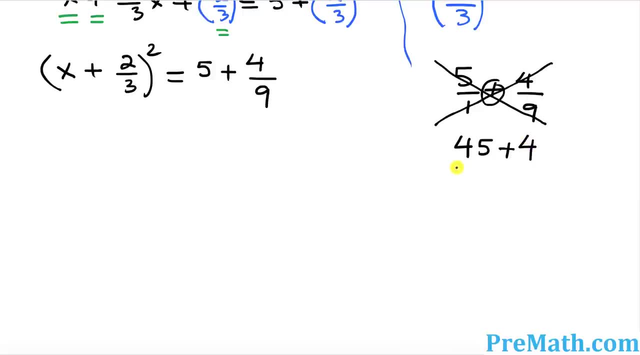 going to be: 4 times 1 is 4 and divided by the bottom numbers, are what 1 and 9. you multiply them 1 times 9 is 9. so 45 plus 4 is what 49 over 9. so this is the. 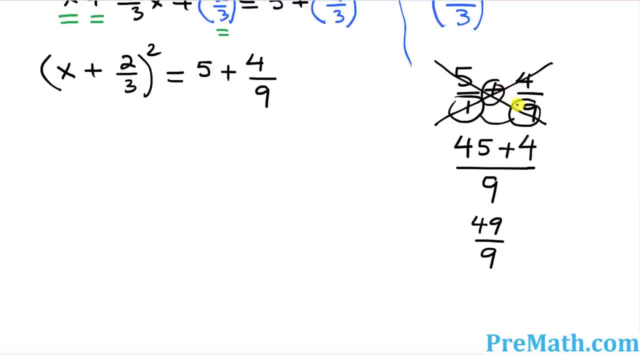 simplest way you can add or subtract any two fractions, and I have already uploaded one of my youtube videos to show this method, so let's go ahead and take care of this thing. so this is what x plus 2 over 3 square, equal to this, adds up to what 49 over 9, the next step we want to. 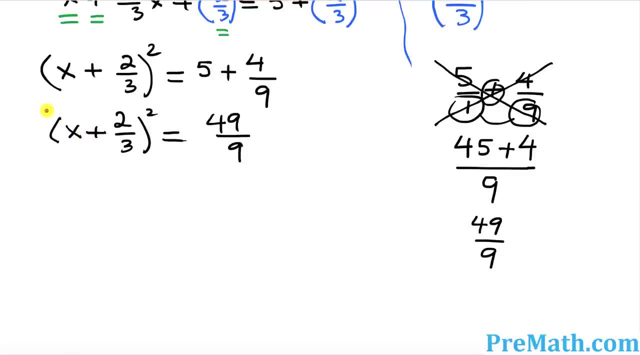 get rid of this square because we want to solve for X. so how to undo this square? we can take the square root on both side. and take the square root on this way, this side as well, and put a plus and minus sign as well. so you can see this square and square root. 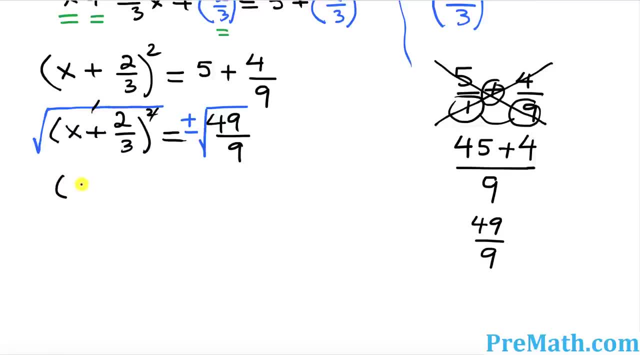 they undo each other. we got what x plus 2 over 3 equals to this: square root of 49 is 7 and the square root of 9 is 3, with a plus or minus sign. now the next. I want you to isolate x, so I'm going to subtract 2. 3rd, from both side, negative 2 over 3. so what happens next is this: 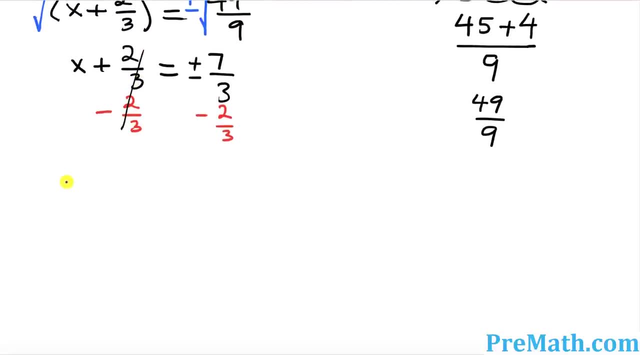 whole thing cancels out. so we got what? x equal to positive or negative, 7 over 3 minus 2 over minus 2, 3. the next thing: I want you to split these positive and negative sign up. so what happens? so this simply become positive 7 over 3 minus 2 over 3 and on. 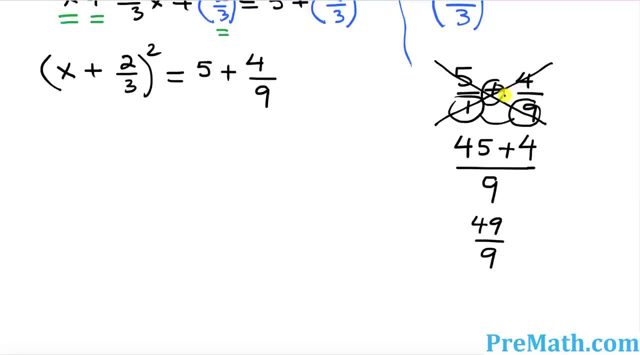 the simplest way you can add or subtract any two fractions, and I have already uploaded one of my YouTube videos to show this method, so let's go ahead and take care of these things. so this is what x plus 2 over 3 square- equal to this, adds up to what 49 over 9. the next. 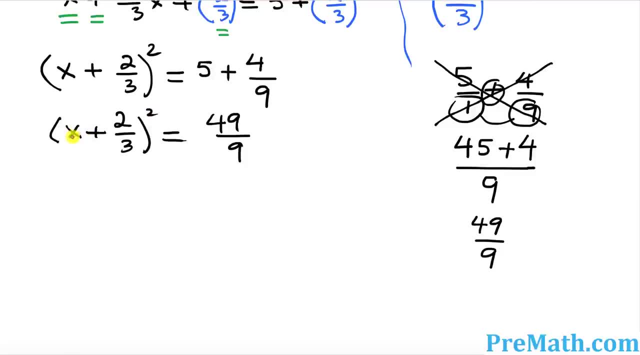 step. we want to get rid of this square because we want to solve for x. so how to undo this square? we can take the square root on both side and take the square route on this side as well, and put a plus and minus sign as well, so you can see this. 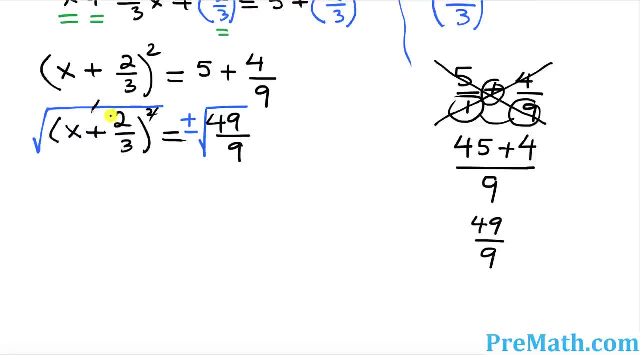 square and square root. they undo each other. we got what X plus 2 over 3 equals to. this: square root of 49 is 7 and the square root of 9 is 3, with the plus or minus sign. now the next. I want you to isolate X, So I'm going to subtract 2. 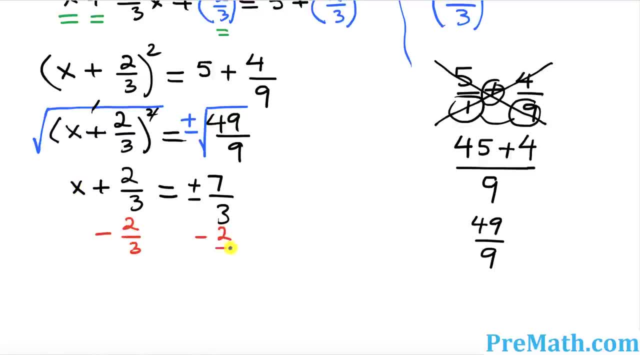 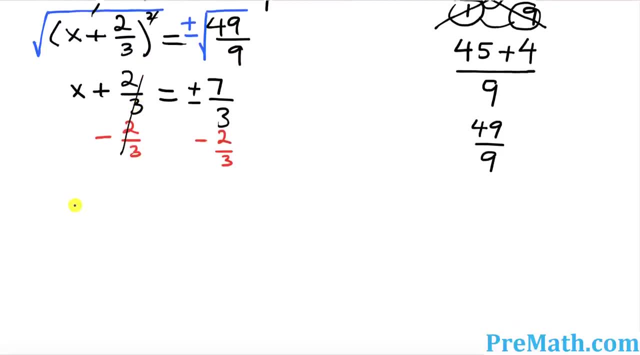 third, from both sides, negative, 2 over 3.. So what happens next is this whole thing cancels out. so we got what? X equal to positive or negative, 7 over 3 minus 2 over 3. the next thing I want you to: 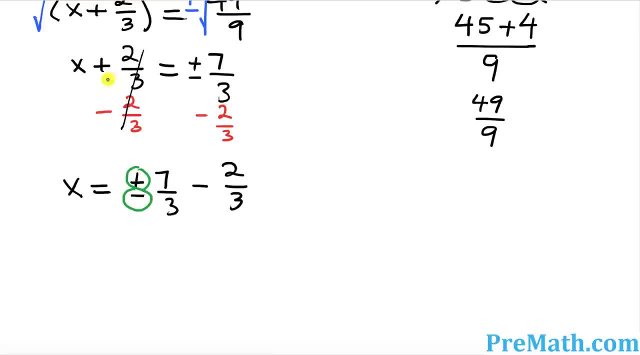 these positive and negative sign up. so what happens? so this simply become positive: 7 over 3 minus 2 over 3, and on this side this is going to be a negative 7 over 3 minus 2 over 3, since we have the common denominator to 3. so I'm going 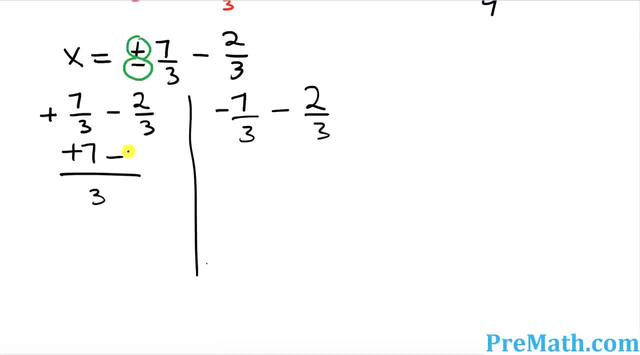 to write down 3 and then this become positive. 7 minus 2 makes what 5 over 3. so our first solution turns out to be: x equals to 5. third and the second solution: we're going to take our 3 at the bottom as a common denominator.